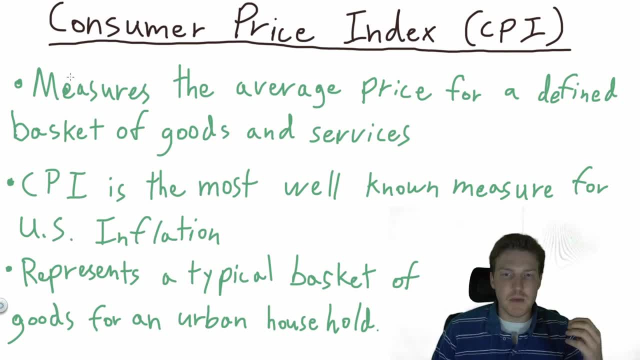 The Consumer Price Index, also known as the CPI, measures the average price for a defined basket of goods or services. This is the most commonly referenced and used measure of inflation in the United States. It's also the measure of inflation that the Federal Reserve uses and calculates. 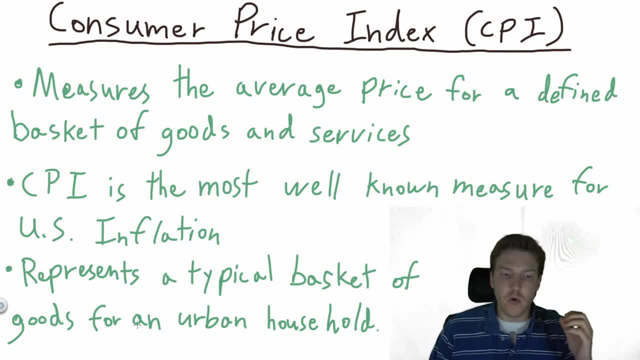 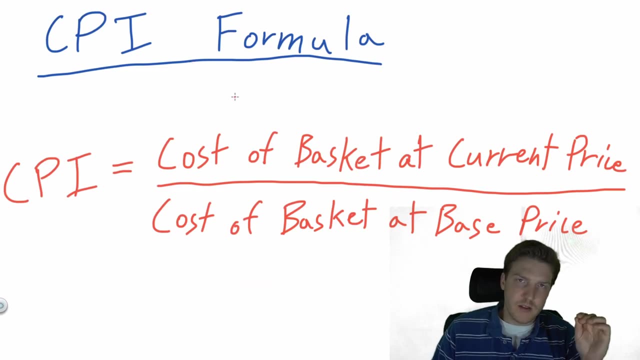 It represents a typical basket of goods for an urban household in the United States, and plenty of other countries have measures of inflation that work similar to CPI. Let's get into how it's calculated. The CPI formula is the cost of a basket of goods at the current price divided. 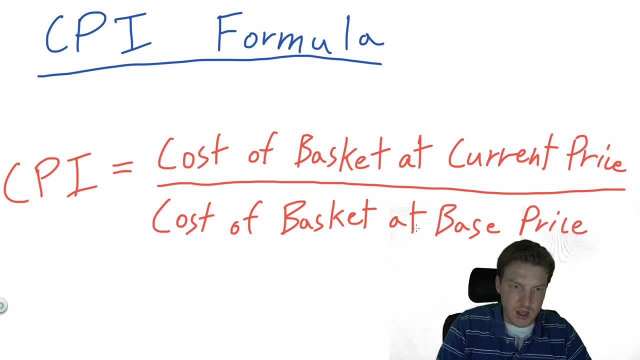 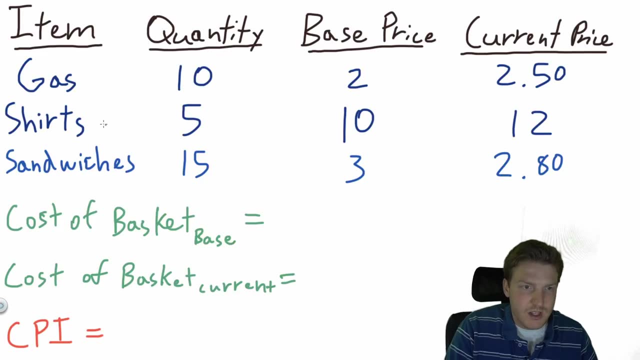 by the cost of the same basket of goods at a base price. If you want to be more technical, you would multiply that calculation by 100.. So let's assume hypothetically that the typical amount of CPI is just divided by the cost of the basket of goods at the current price. 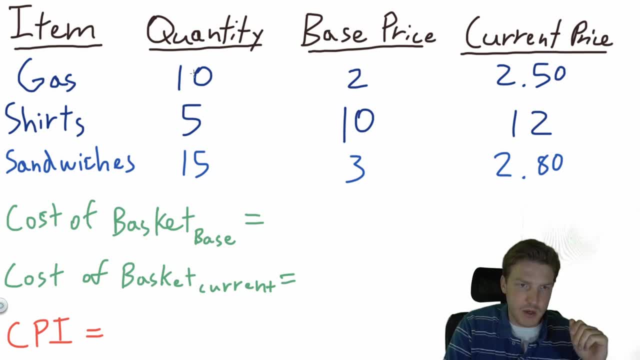 And you'd multiply that calculation by 100.. So let's assume hypothetically, that the typical amount American family buys this simplified basket of goods. So they're going to buy $10, or no, they're going to buy 10 gallons of gasoline, five shirts and 15 sandwiches, And let's say, at a base, 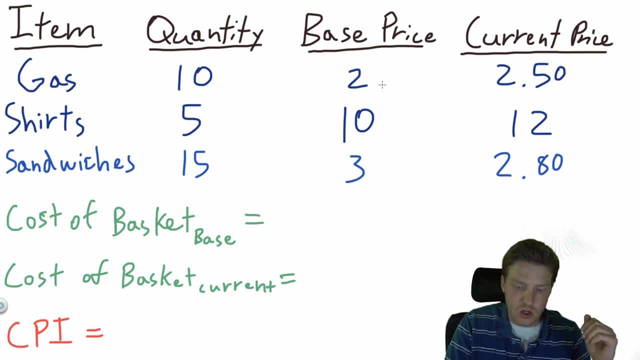 price. so let's say one year ago a gallon of gasoline used to cost $2.. Now that same gallon of gasoline costs $2.50 today. And let's say, the shirt used to cost $10.. Now today it costs $12.. 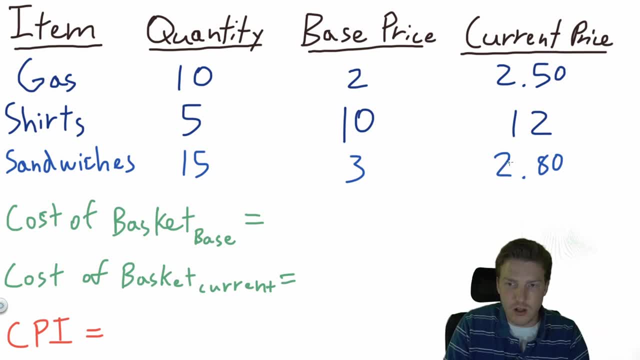 And the sandwich used to cost $3. Now today it costs $2.80.. So first we're going to calculate the cost of a basket at the base prices, right? So that's just going to be $10, or 10 gallons of. 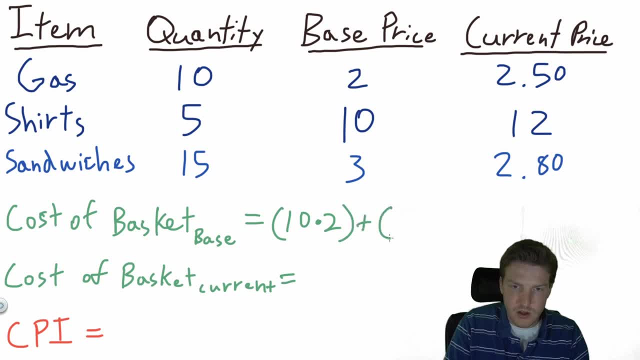 gasoline times $2, plus five shirts times $10, plus 15 sandwiches. multiplied by $3 per sandwich, That's going to give us a value of $115 for the base index. Now we're going to calculate the cost of a basket at the base price. So let's say a $10, or 10 gallons. 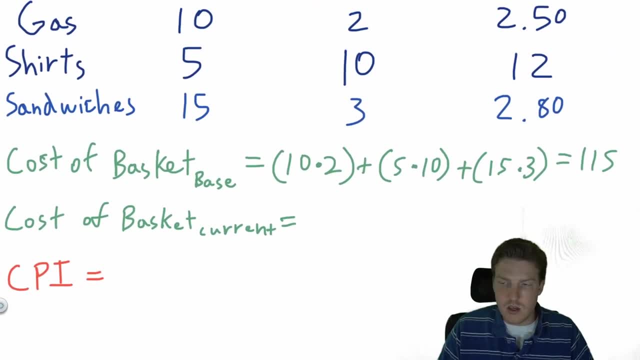 of gasoline used to cost $2.. Now, today we're going to calculate the cost of a basket at the current prices. okay, So it's going to be still the same: 10 gallons of gasoline, but now it's going to be $2.50 a gallon. And then it's also going to be five shirts, but now the shirts cost.